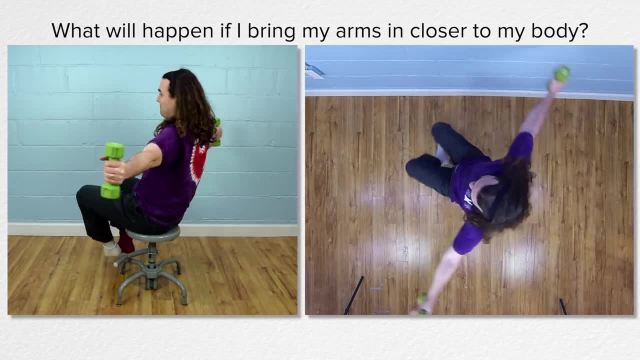 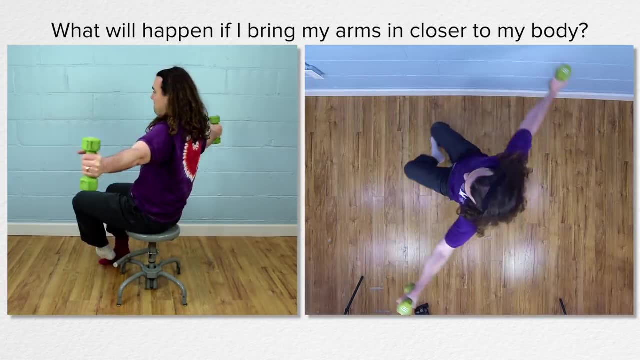 I feel like I've seen something like this before. Yeah, it's just like when a figure skater brings their arms in while spinning, Or a gymnast Or a diver Or a dancer, Sure, but what happens? Oh, a bringing your arms in. 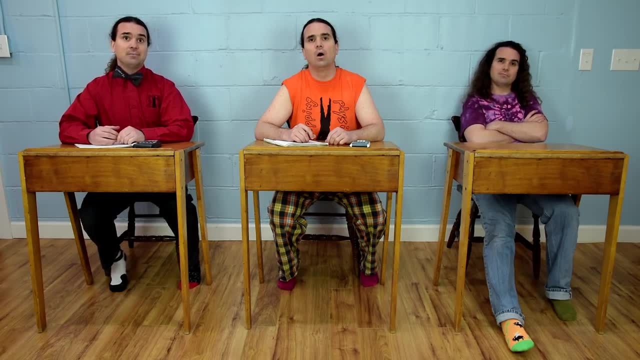 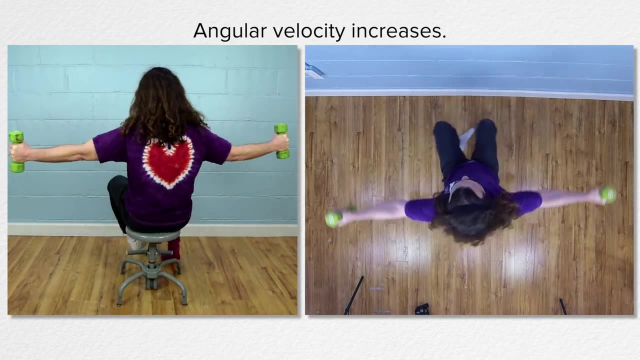 Your arms in will increase your angular velocity. right, That is correct. When I bring my arms in closer to my body, the angular velocity of the stool and me increases. But the question is why? Why does bringing my arms and the two masses in closer to my body? 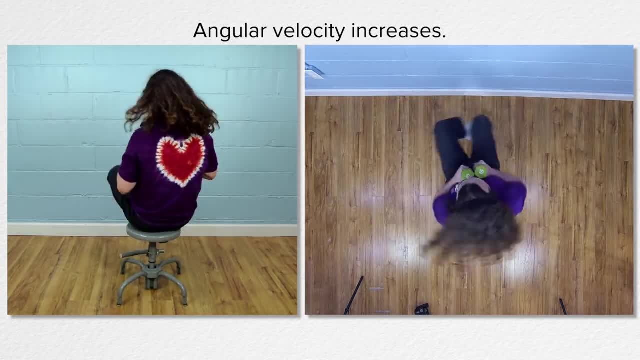 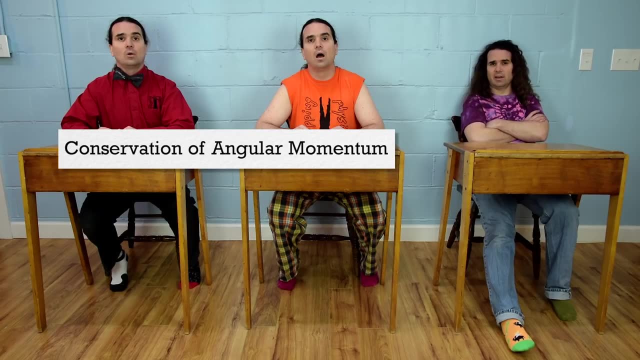 increase the angular velocity of the system. Can we assume the angular momentum of the system is conserved? Yes, we may assume angular momentum is conserved in this example. Well then, the initial angular momentum of the system equals the final angular momentum of the system. 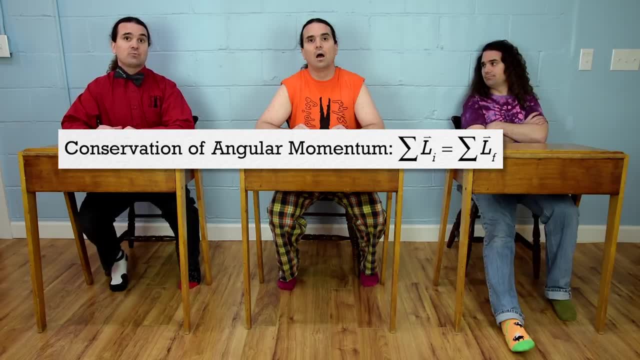 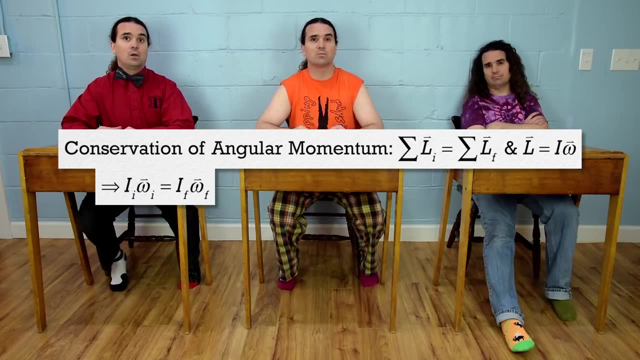 And angular momentum of a rigid object with shape equals rotational inertia times angular velocity. So rotational inertia initial times angular velocity, initial equals rotational inertia final times angular velocity final. Oh, yeah, yeah. So rotational inertia of a system of particles equals the sum of the mass of each particle. 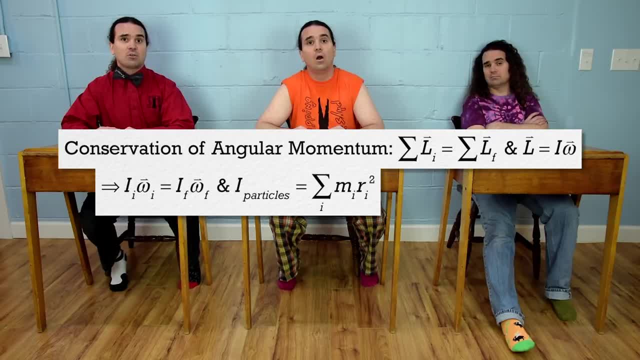 times the square of the distance each particle is from the axis of rotation, or r squared. Bringing in your arms decreases the average distance. everything is from the axis of rotation, which decreases the rotational inertia. And if the rotational inertia is decreased, the angular velocity must increase. 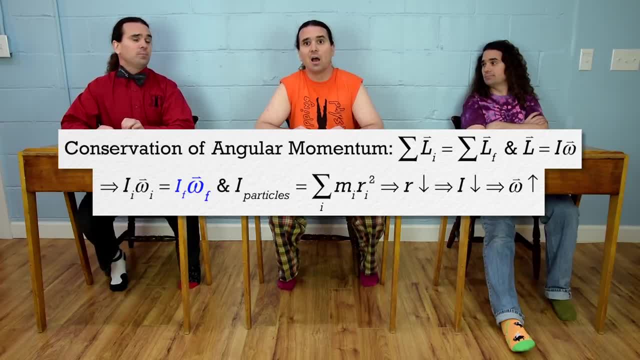 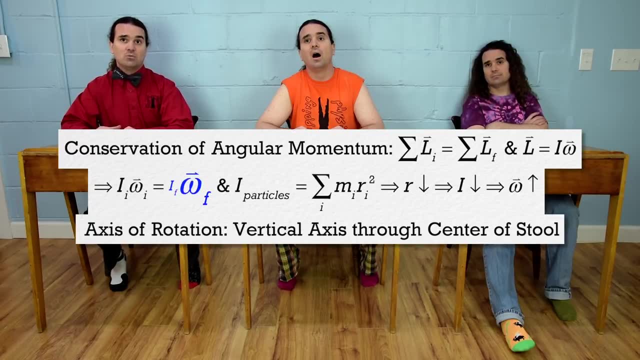 to keep the angular momentum of the system constant. You know. I just want to specifically point out that the axis of rotation is the vertical axis which passes through the center of the stool. We always have to define the axis of rotation when talking about rotational inertia and angular momentum. 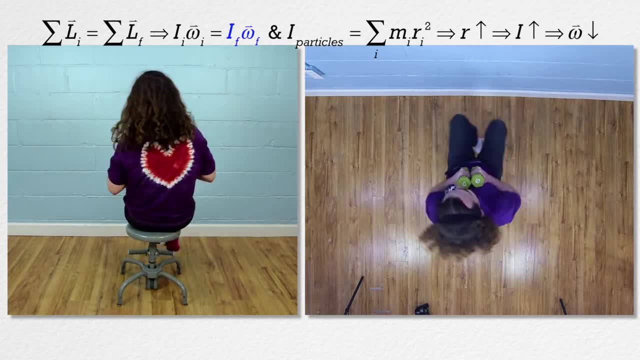 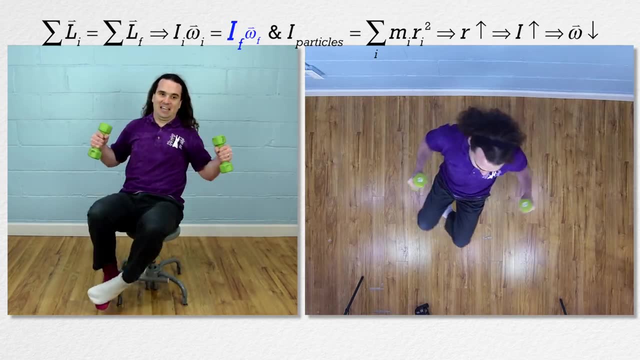 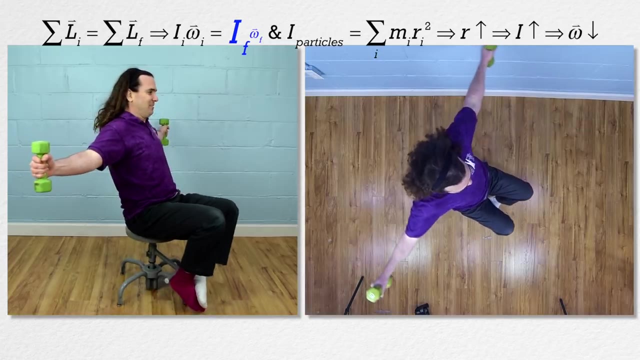 Very nice And notice. the reverse is also true. Moving the masses from close to the axis of rotation to farther from the axis of rotation increases the average distance each object is from the axis of rotation, increasing the rotational inertia of the system and the angular velocity of the system must decrease. 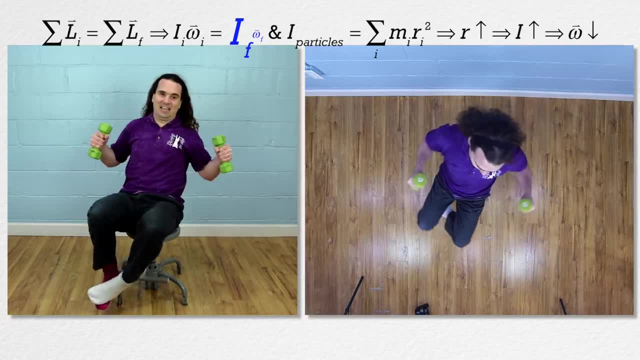 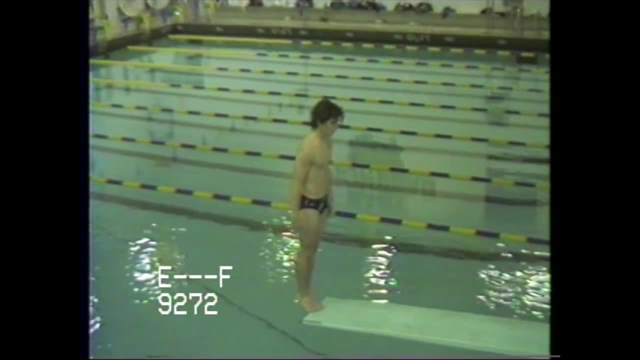 to maintain a constant angular momentum of the system. As was pointed out earlier, conservation of angular momentum occurs in many sports. For example, this is me diving in high school a couple of years ago. I am doing an inward one-and-a-half tuck. 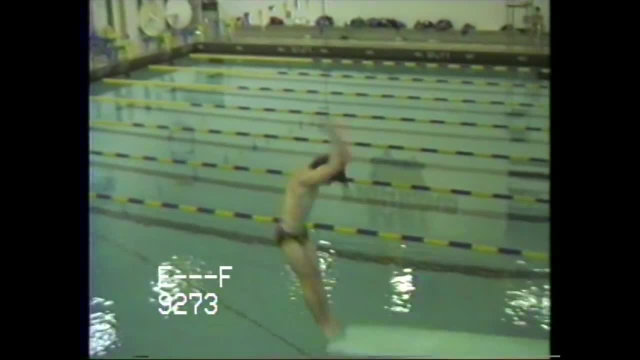 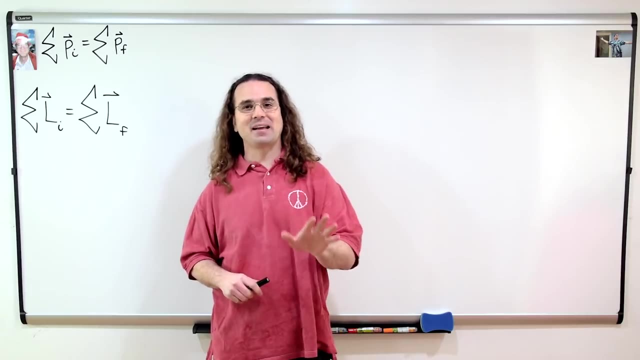 Wait a second. That's you in high school. Yes, That is me during my 10th grade year of high school. Oh, wow, Okay, Yeah, okay. So let's get back to physics As I leave the board and go into the air. 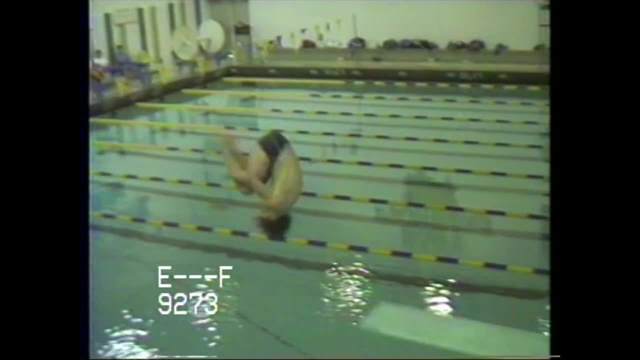 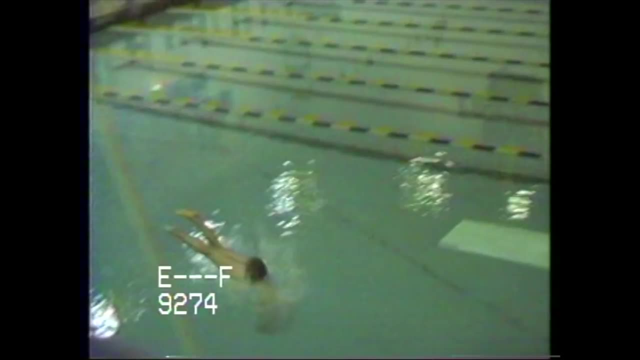 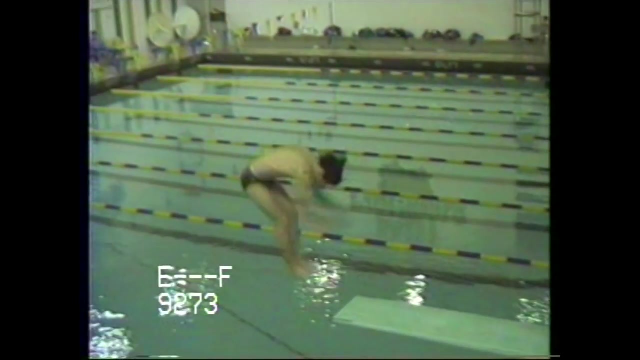 I pull my legs and arms in to form the tuck position. This decreases the rotational inertia of my body considerably and therefore increases my body's angular velocity, And while I'm in the air, angular momentum is conserved When I am almost done with one-and-a-half rotations. 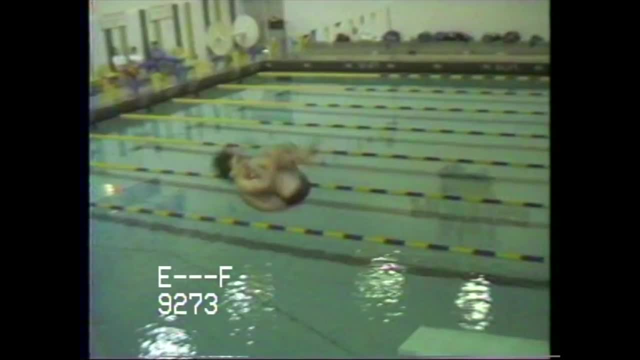 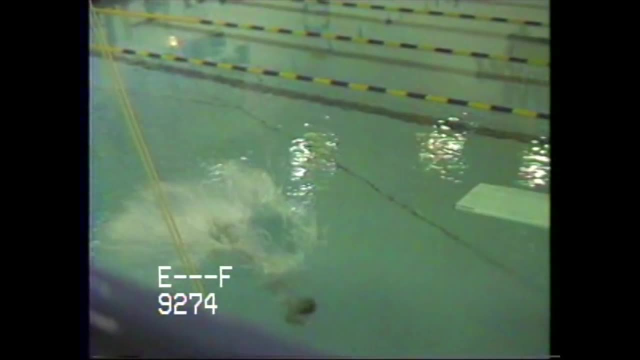 I straighten my body to increase my rotational inertia and decrease my angular velocity. This is similar to moving my arms on the stool, like we just demonstrated. Now let's talk about when angular momentum is conserved, But first remind me, Billy. 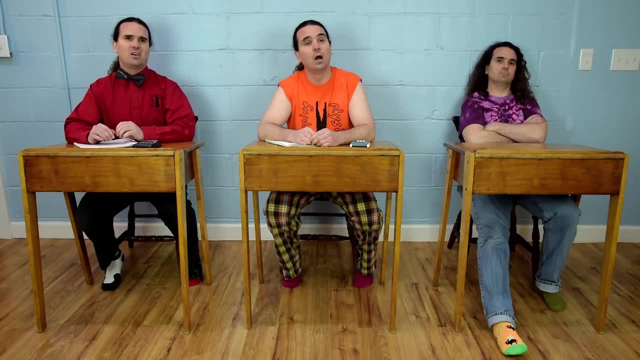 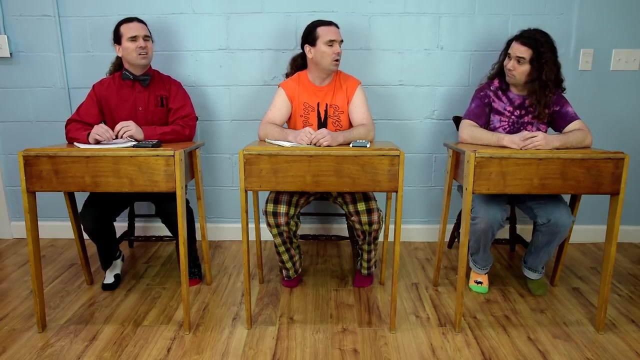 when is linear momentum conserved? Um, Okay, so remember you start with Newton's second law: Net force equals mass times acceleration. No, Actually it starts with the version of Newton's second law that has linear momentum in it. Okay, 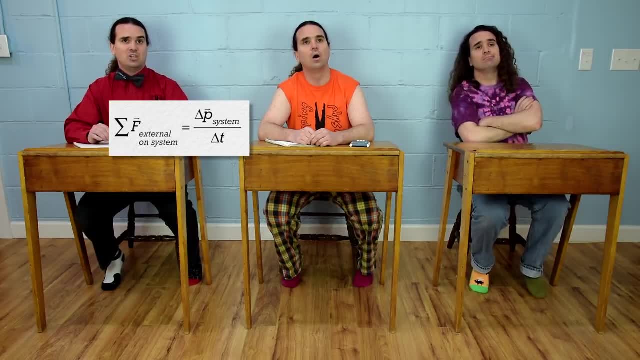 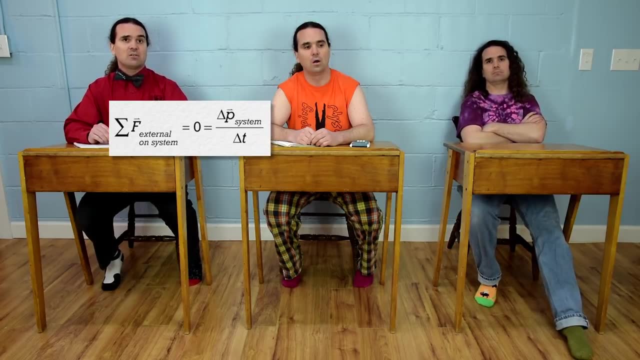 So the net external force on the system equals change in linear momentum over change in time, And linear momentum is conserved when the net force acting on the system equals zero. So multiply both sides by change in time. Change in time cancels out and we are left with 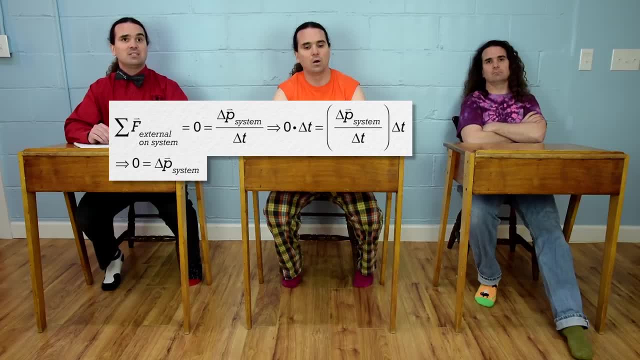 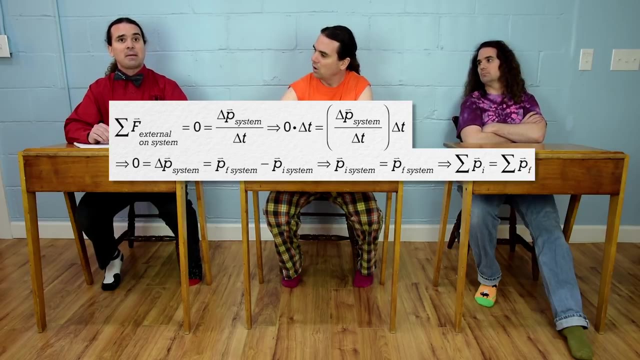 zero equals the change in linear momentum of the system. Change in linear momentum equals the final linear momentum minus the initial linear momentum. Add initial linear momentum of the system to both sides and we get the initial linear momentum of the system equals the final linear momentum of the system. 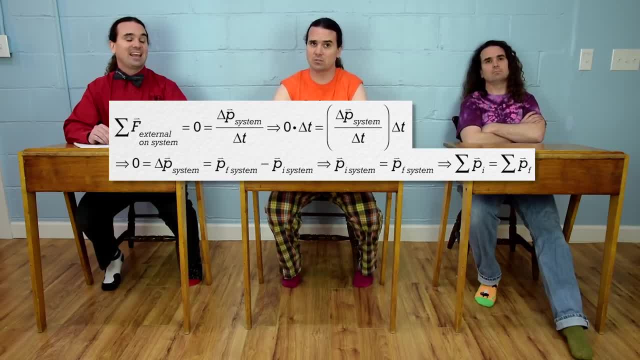 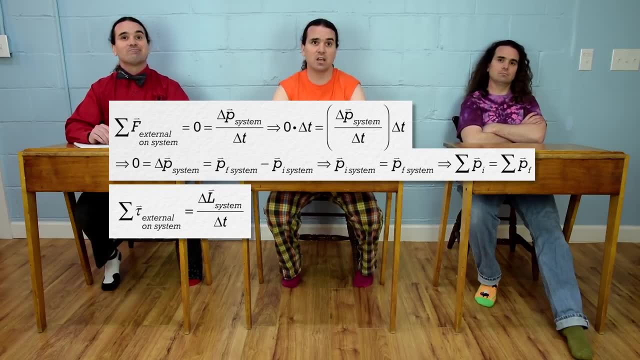 Then conservation of angular momentum should use the rotational form of Newton's second law. The net external torque acting on the system equals change in angular momentum over change in time, And angular momentum should be conserved when the net external torque acting on the system equals zero. 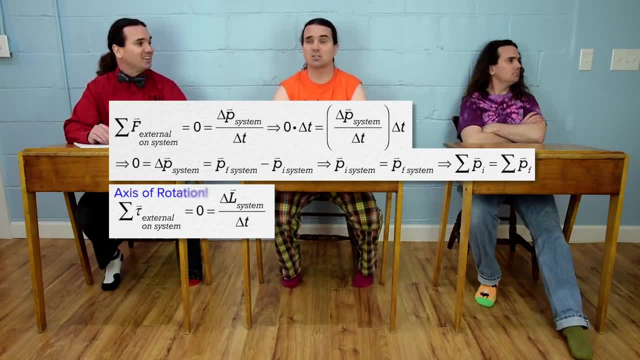 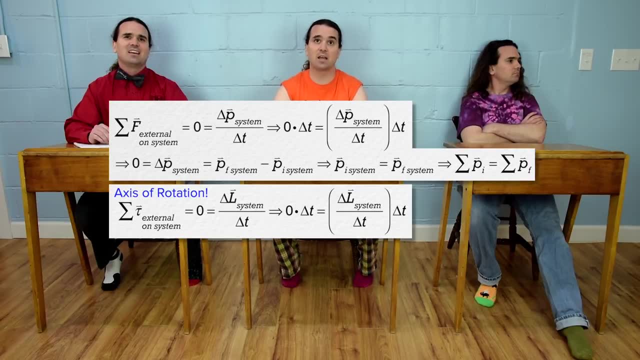 And we need to identify the axis of rotation. We've got to make sure we do that. Then we can multiply both sides by change in time. Change in time cancels out and we are left with zero. equals the change in angular momentum of the system. 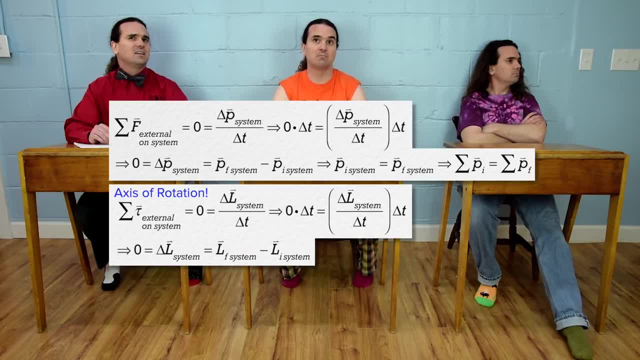 Change in angular momentum equals final angular momentum minus initial angular momentum. Add angular momentum of the system to both sides and we get the initial angular momentum of the system equals the final angular momentum of the system. All you did was pretty much say what I said. 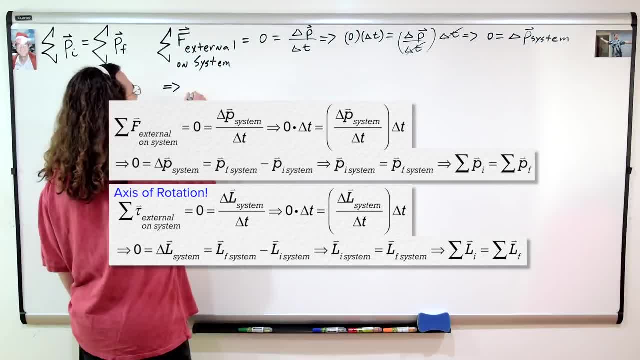 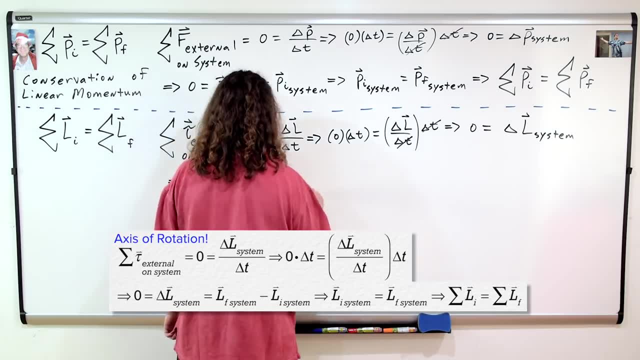 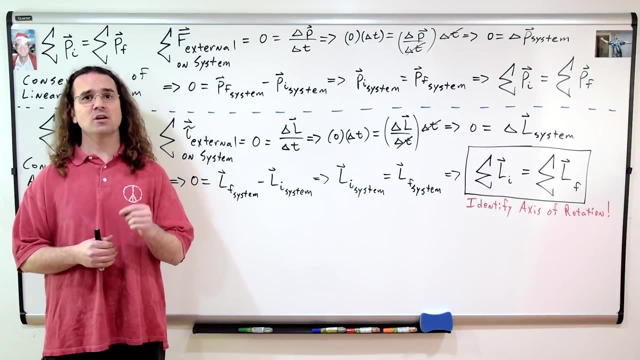 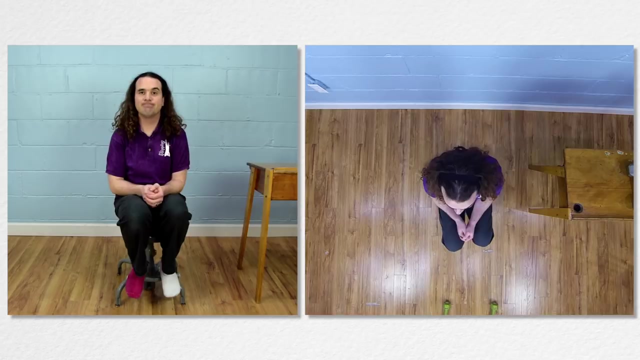 only with angular instead of linear. Yep, that's what I did, Bobby. you are correct that angular momentum is conserved when the net external torque acting on the system equals zero. To demonstrate this, let's return back to me on the stool. 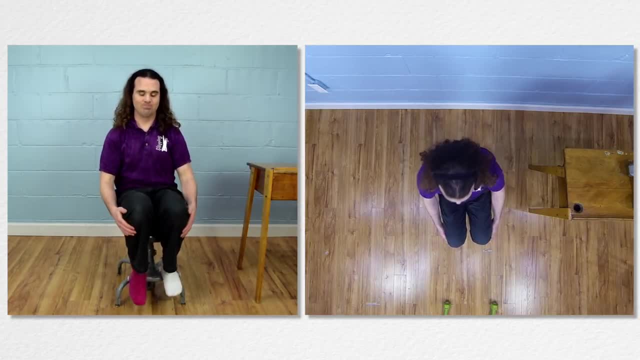 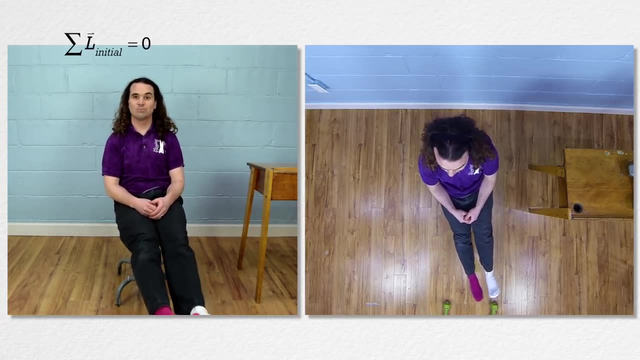 While I am just sitting there class. what is the angular momentum of the Mr P and stool system? Zero, Because you have zero angular velocity. And if I do not apply a force on anything, do you see how the net external torque? 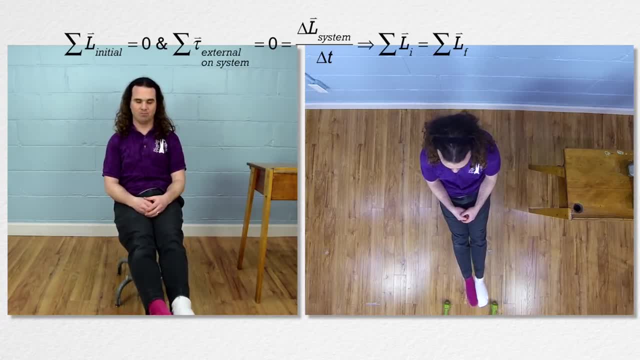 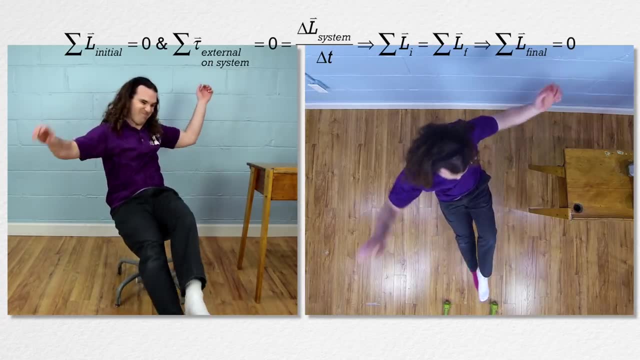 acting on the stool and me will be zero. Yes, Alright, so the angular momentum of you and the stool will stay equal to zero. Exactly, Bo. Which is why, no matter how much I wave my arms and legs about, I cannot change the angular momentum of the system. 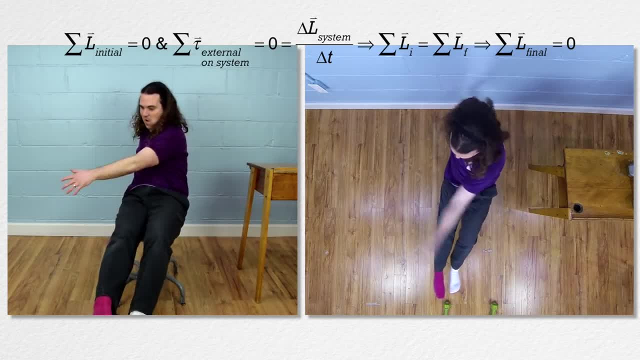 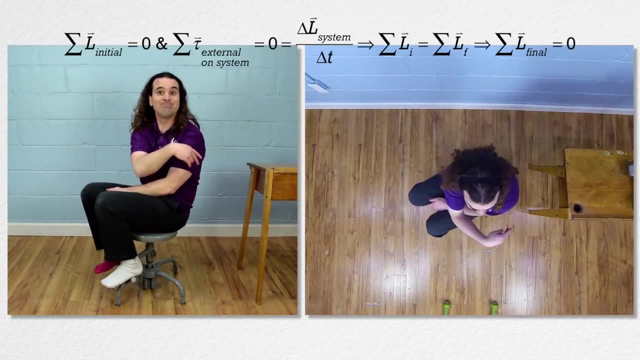 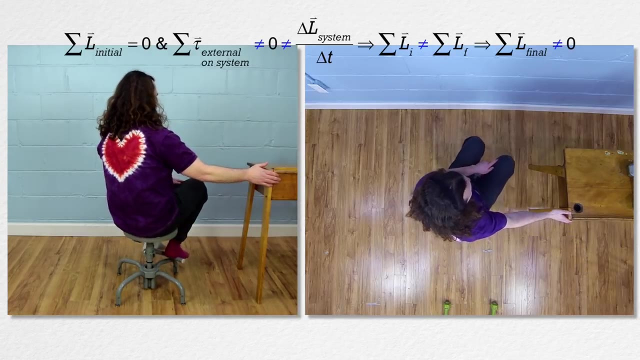 and the angular velocity of the system remains equal to zero. However, if I simply push off of something, the object, which is external to the system, applies a net external torque to the system and the stool and I begin to rotate because angular momentum is no longer conserved. 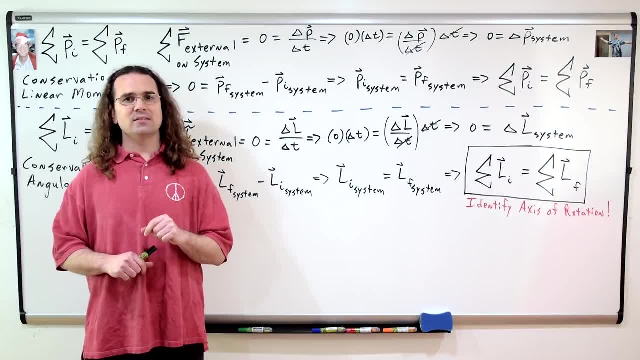 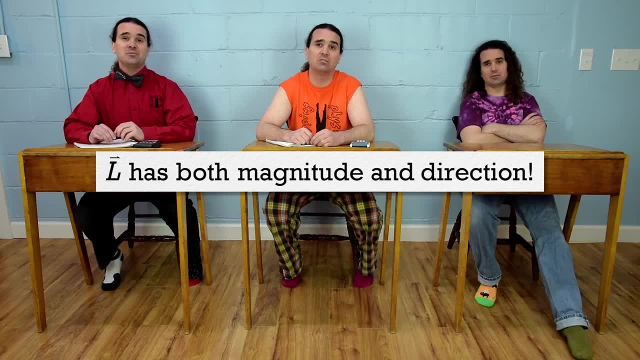 Okay, that's cool. Okay, I want to talk for a bit about the fact that angular momentum is a vector, which means class. angular momentum has both magnitude and direction. Therefore, when we look at this top, which is rotating clockwise, when viewed from above, 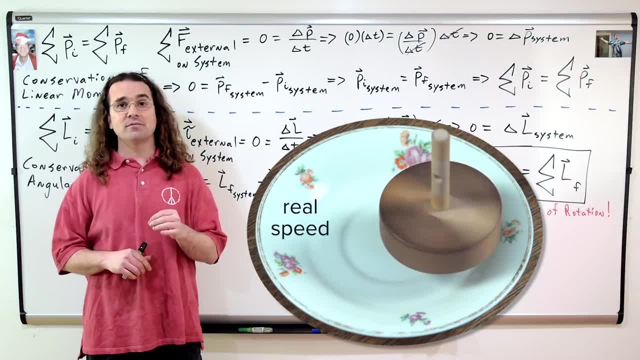 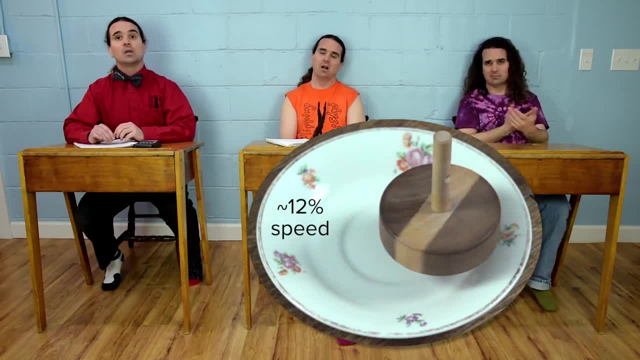 Bo, what is the direction of the angular momentum of the spinning top? We still use the right-hand rule to find the direction of the angular momentum right? Yes, absolutely, We use the right-hand rule. Okay, so I take my right hand, curl my fingers. 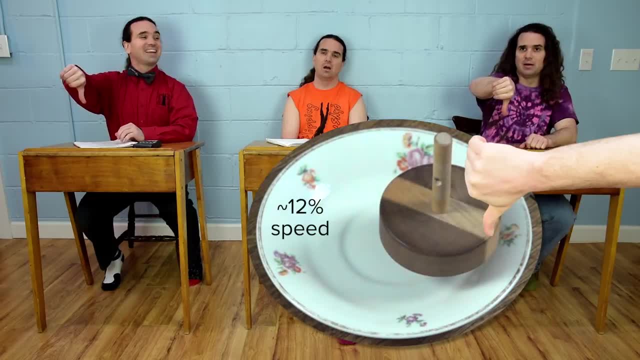 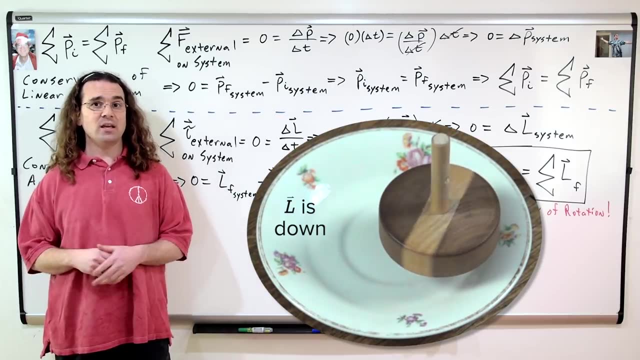 in the direction the top is spinning, and stick out my thumb. My thumb points down, so the angular momentum of the spinning top is down. That is correct. And just like an object will tend to maintain its linear momentum, an object will also tend to maintain.